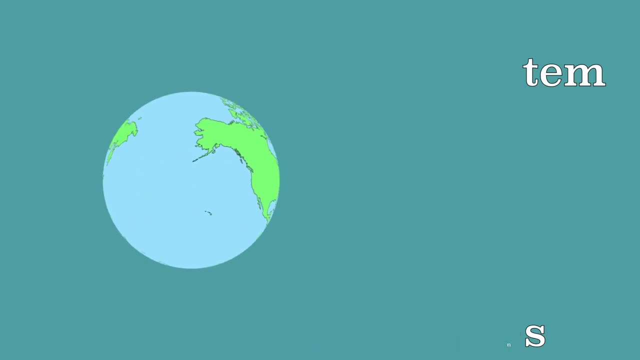 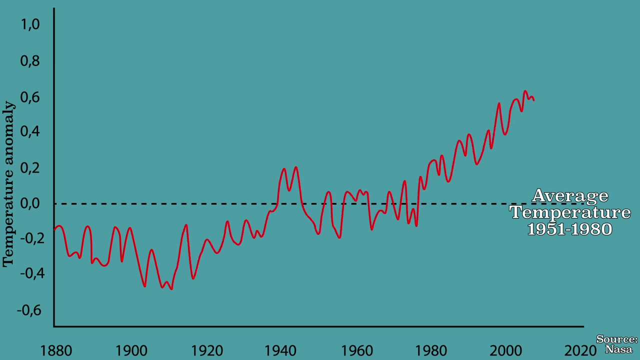 In previous videos, you have already learned that the climate has always changed during Earth's history and was caused by natural variations. However, global warming accelerated very fast in recent decades. Many scientists agree that people have caused this climate change through greenhouse gas emissions. But what are the consequences of this climate? 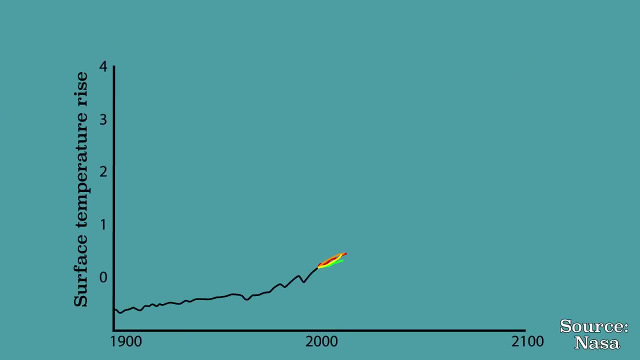 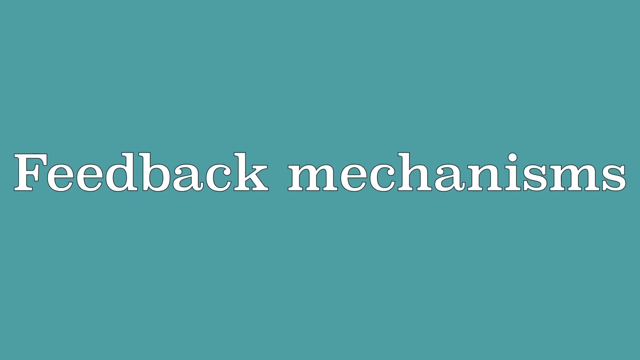 change. How climate change will develop is still difficult to estimate. Future expectations often vary widely. The Earth also reacts to the increase of CO2 in the atmosphere and the temperature rise at the surface. This response is called a feedback mechanism. Some feedback mechanisms enhance global warming and are therefore called positive feedback. 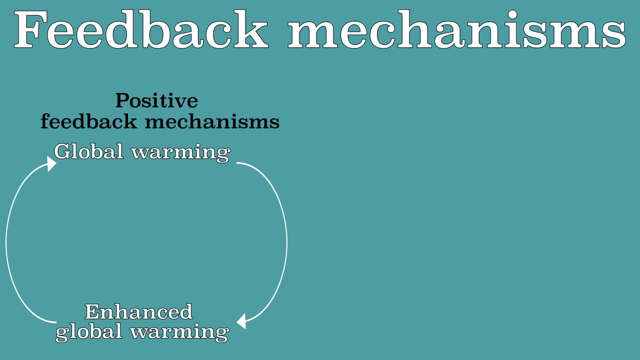 mechanisms. These are not called positive feedback mechanisms because we like them, but they are called positive because they enhance the first effect of warming. There are also processes that counteract global warming. These are therefore called negative feedback mechanisms because the first effect of global warming is negative. 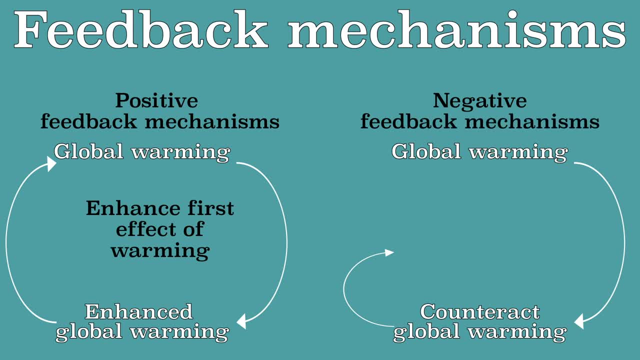 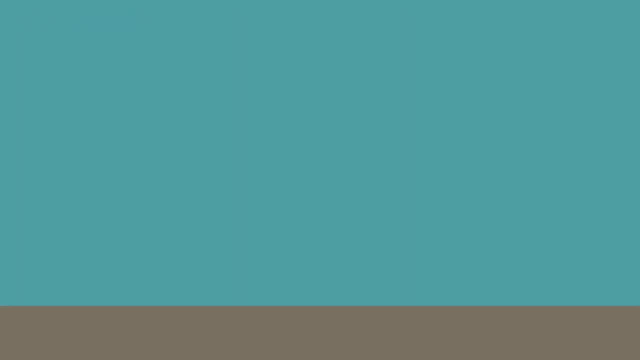 because the first effect of warming is actually counteracted. The Earth has a lot of feedback mechanisms of which it is not yet completely clear how they work, and that makes it unclear how exactly the Earth reacts to current global warming. A fairly clear feedback mechanism is the albedo effect. 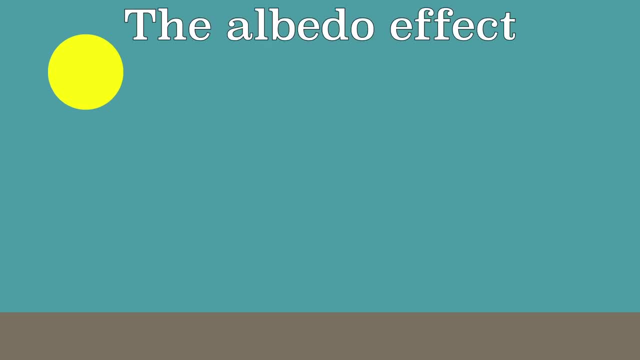 The albedo is the degree of reflection of solar radiation from an object. Fresh snow reflects about 90% of the sun's energy and thus has a cooling effect on the Earth. When it gets warmer, more snow melts. As a result, less warmth of the sun is reflected and therefore it can get warmer, so that more 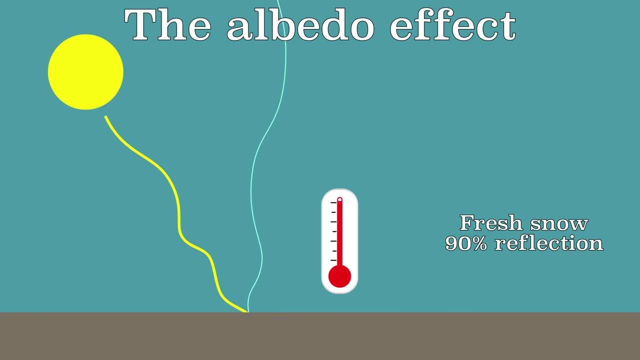 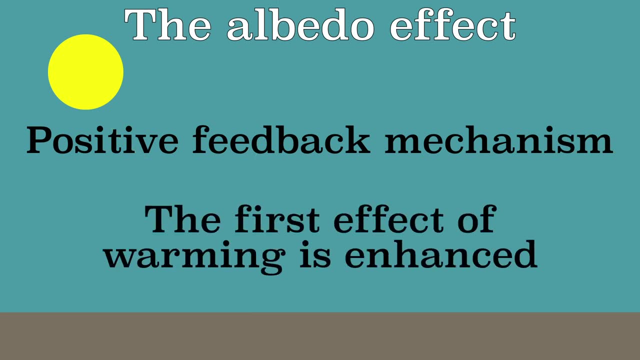 snow can melt. So this is a clear example of positive feedback. The first effect of warming is amplified. This is an important feedback mechanism. in the cycles of Milankovitch You have already learned that he found out that the position of the Earth relative to 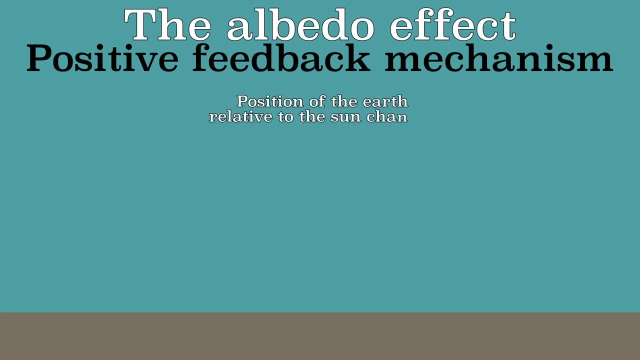 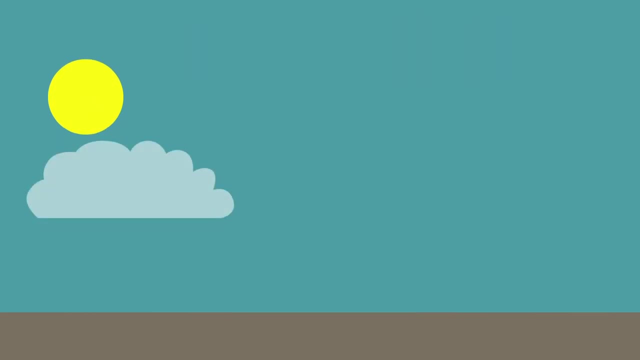 the sun can make it slightly warmer or colder on Earth. When the soil gets a little colder, snow can accumulate, reflecting more heat and cooling the Earth even more, and create an ice age. A more unclear feedback mechanism is, for example, cloud formation.